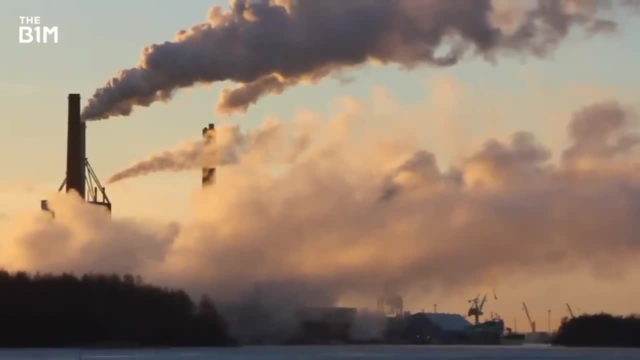 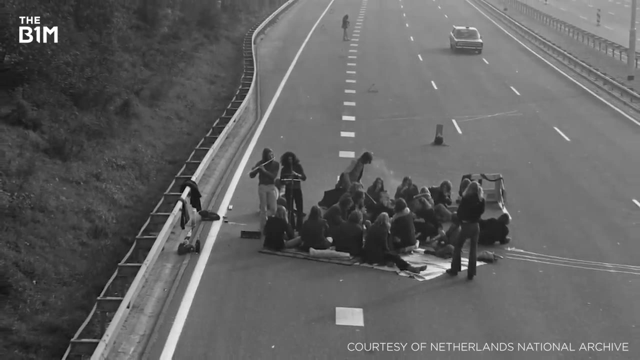 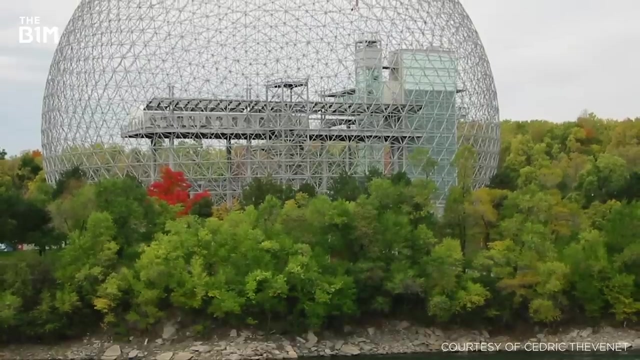 The current revival of green architecture began in the 1970s, when the energy crisis, coupled with growing awareness of humankind's impact on the environment, propelled architects and engineers to think more carefully about sustainable development. Although there are many different ways to approach sustainable building design, an increasing number of architects and engineers 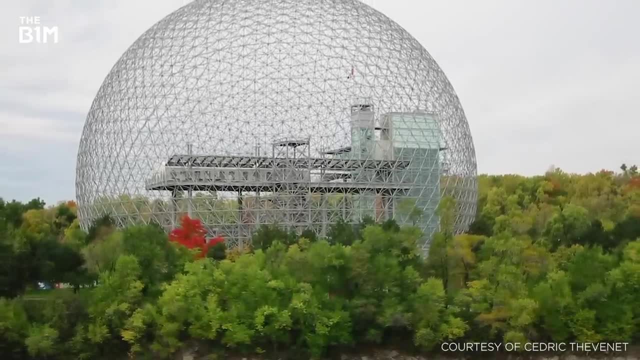 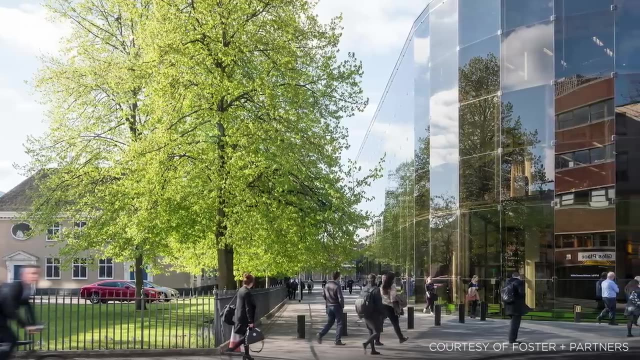 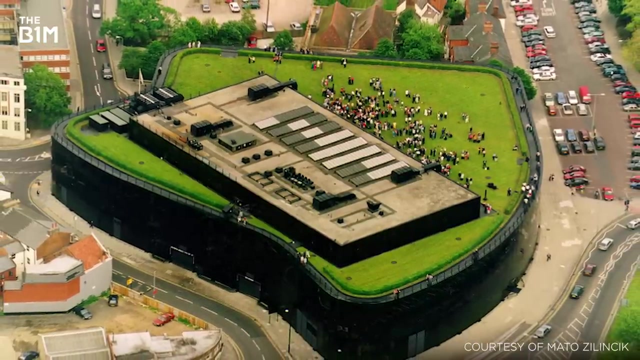 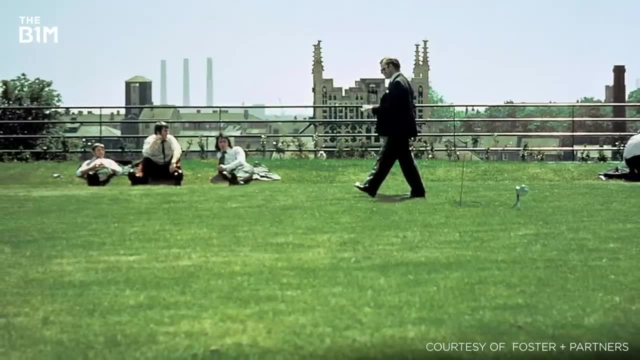 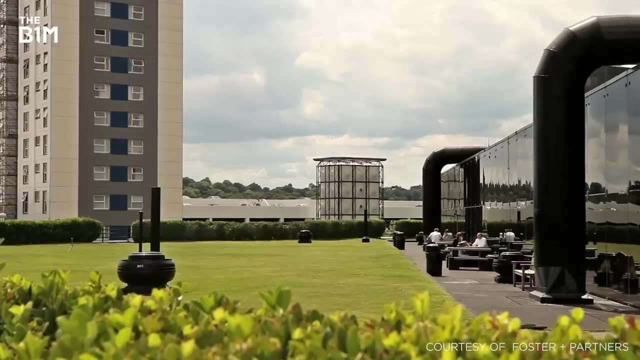 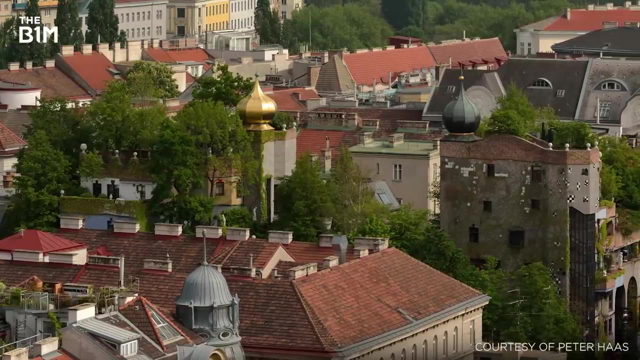 which could be used as a breakout space for the firm's employees. Other approaches advocate integrating trees and plants within buildings, often to soften the psychological impact of living in modern cities. One of the most idiosyncratic proponents of this approach was Austrian artist Friedensreich. 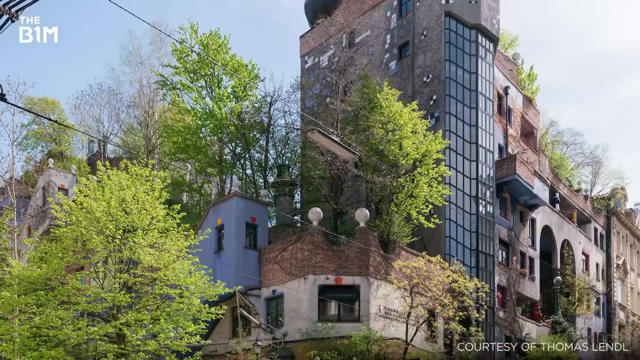 Hundertwasser, who designed an apartment building and a number of hotels throughout the 1980s and 1990s, incorporating mature trees in view of the effects of climate change. Hundertwasser, who designed an apartment building and a number of hotels throughout the 1980s and 1990s. incorporating mature trees in view of the effects of climate change. Hundertwasser, who designed an apartment building and a number of hotels throughout the 1980s and 1990s, including a number of hotels throughout the 1980s and 1990s. 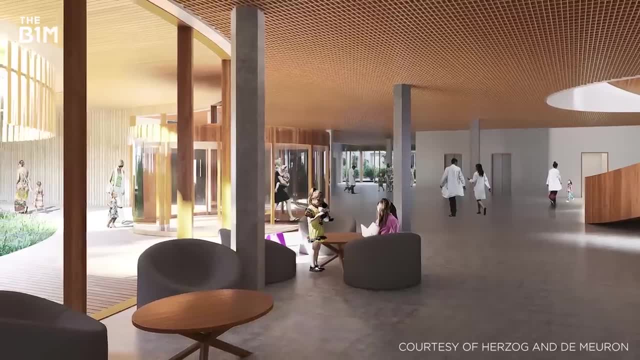 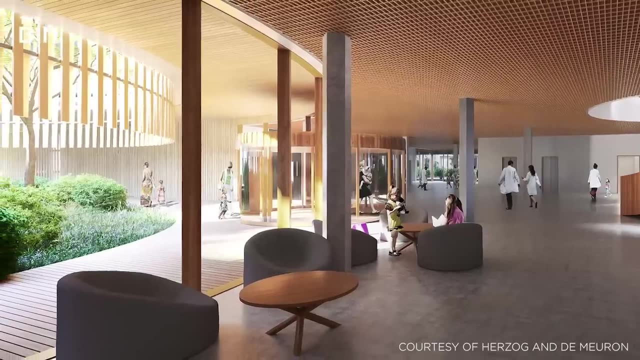 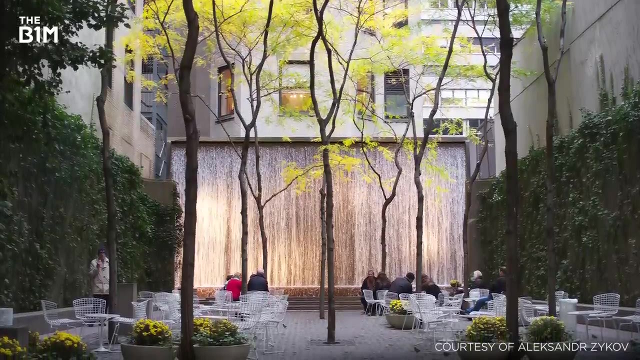 including a number of hotels throughout the 1980s and 1990s. Since then, research has demonstrated that green space can have a substantial physical and psychological impact on our urban environments. Studies have shown that even a small park can reduce local surface temperatures by as much. 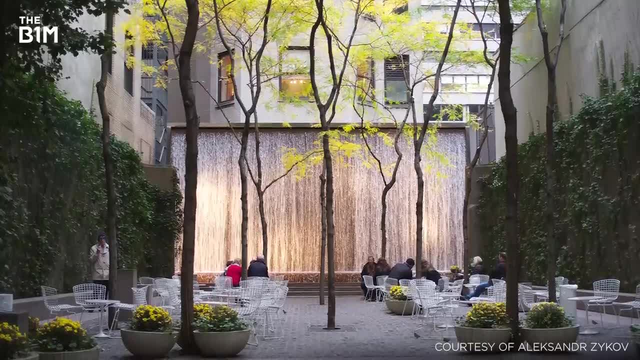 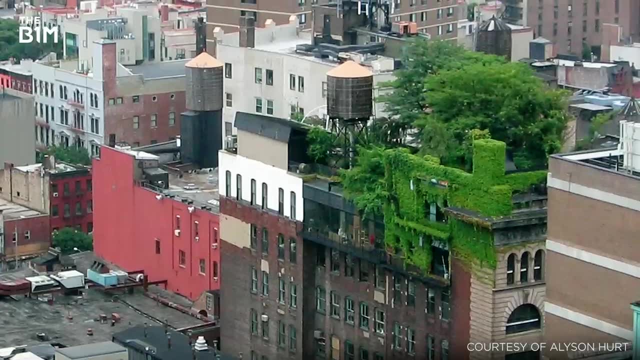 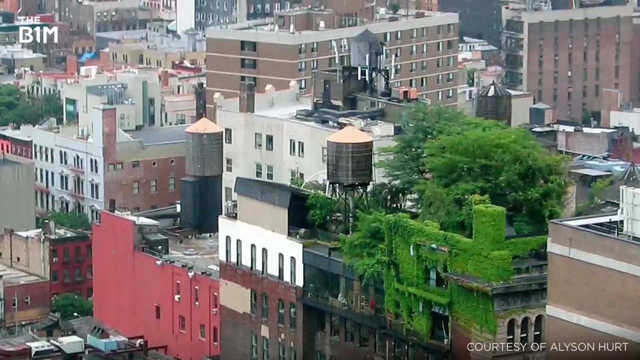 as 7 degrees Celsius, while urban trees planted along streets can reduce temperatures by up to 3.9 degrees Celcius. Green roofs also perform well. Their temperatures can be as much as 4.4°C cooler than conventional roof finishes and, if used across an urban area, could reduce temperatures by as much. 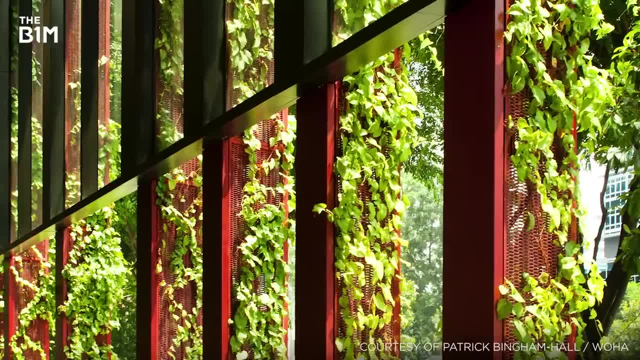 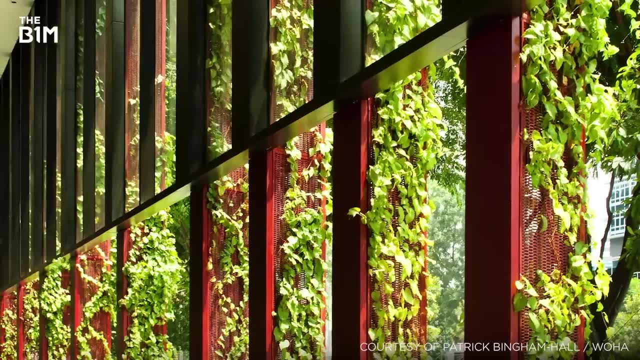 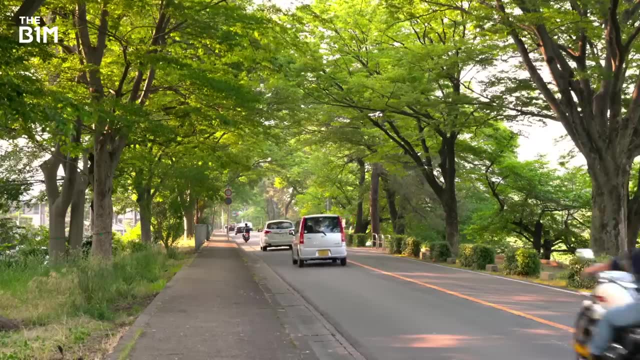 as 7°C. The benefits of temperature regulation can also be found in deciduous trees, which offer passive solar shading in the summer, while allowing the sun's rays to penetrate deep into a building's floorplan during winter months. Trees can also reduce the amount of exhaust gases and particles in the air. with some 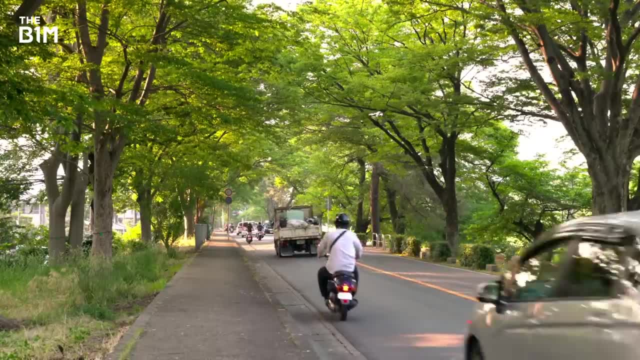 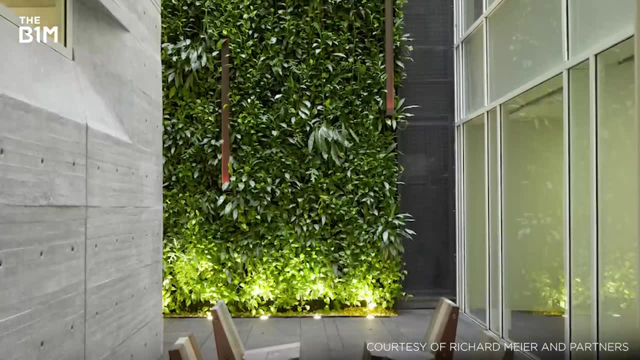 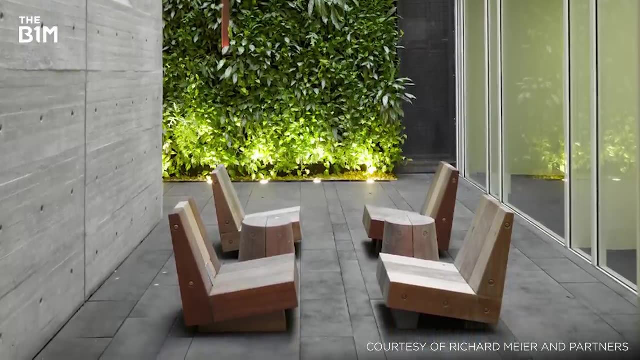 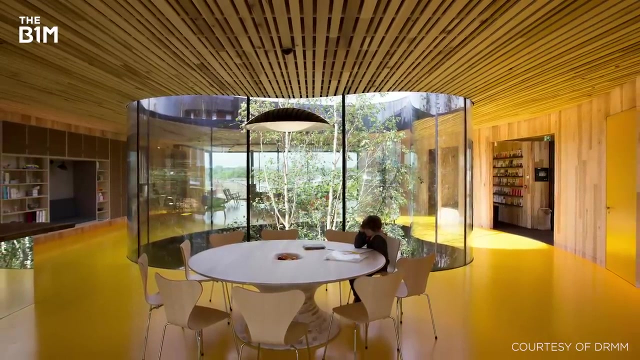 studies claiming they help reduce local concentrations of nitrogen oxide by up to 57%. Aside from their physical impact, there is powerful evidence that the inclusion of plants within our built environment can deliver psychological benefits too. Hospital patients with views of green spaces have had faster recovery times, and plants have been shown to reduce stress. 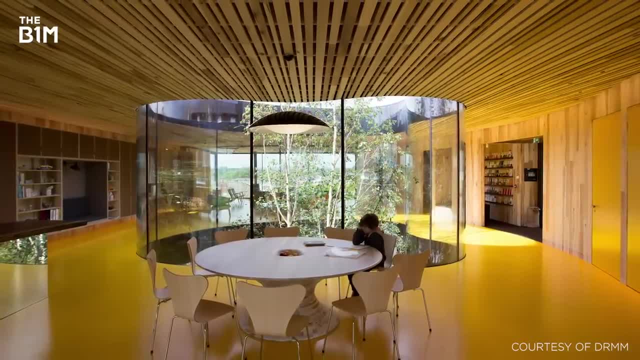 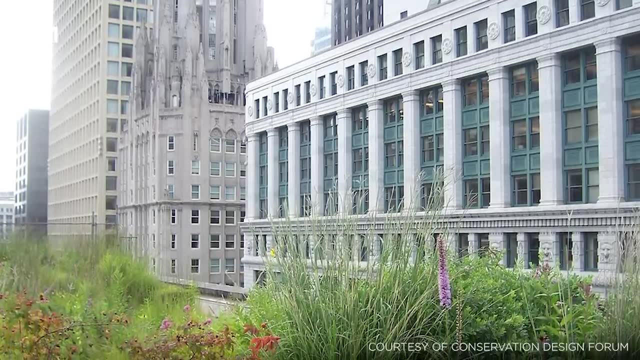 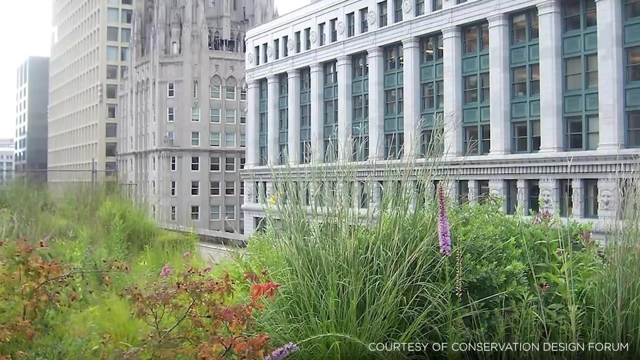 amongst office workers, which, in turn, increases their productivity. This can often lead to extensive planting being added to existing structures, either as a way to replace lost habitats or decrease urban heat island effects, or to create green spaces for the benefit of people living and working in dense urban areas. 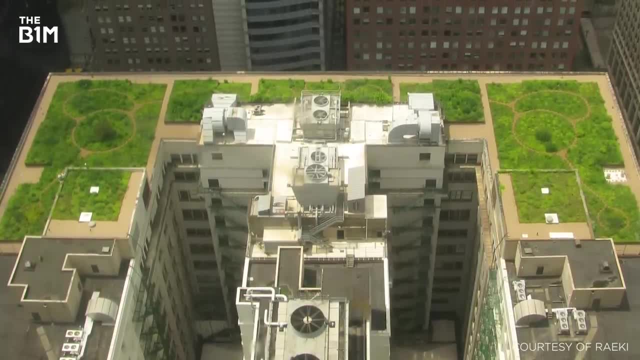 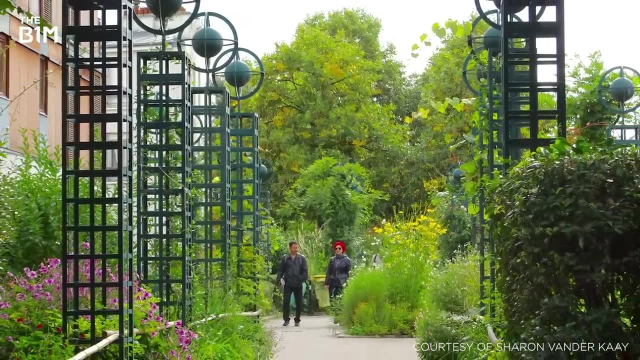 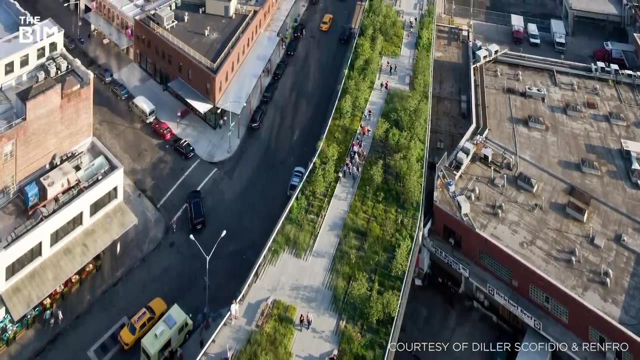 Projects of this kind include Chicago's Green Roofs project, launched in 2001,, as well as linear parks such as the 1993 Promenade Plantée in Paris. This was the precursor to the hugely popular High Line that now occupies a disused elevated 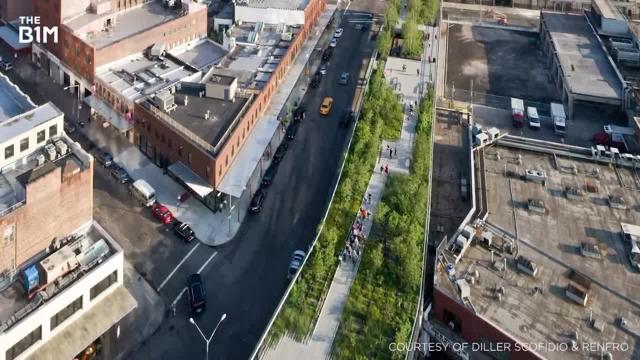 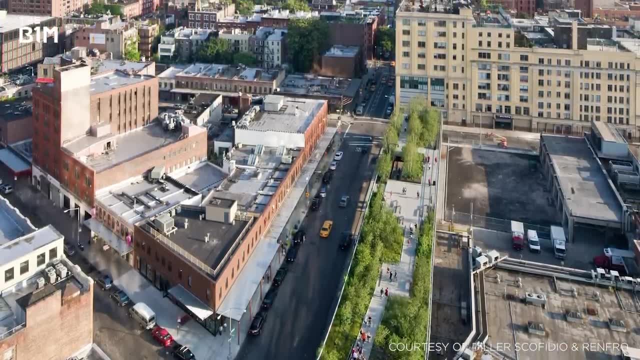 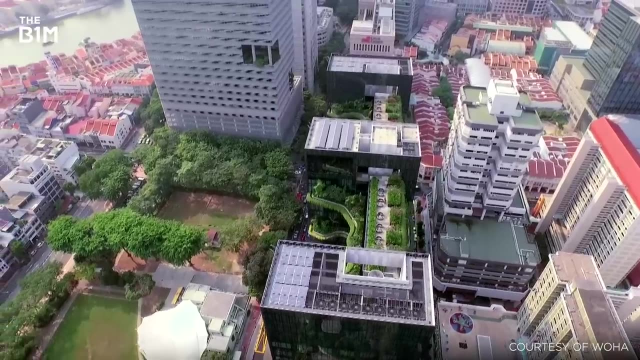 freight railway in Manhattan, which first opened in 2009,. and Thomas Heatherwick's unrealised Garden Bridge in London, proposed in 2013.. Conclusion, Conclusion, Conclusion. The Green Roof project is the growing trend of integrating entire trees into built structures, leading to increasingly ambitious projects with deep, strategically placed planters that 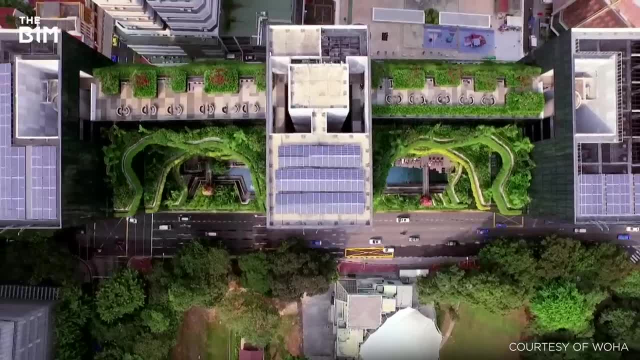 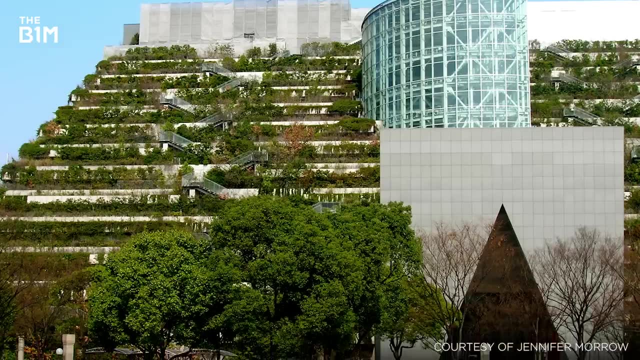 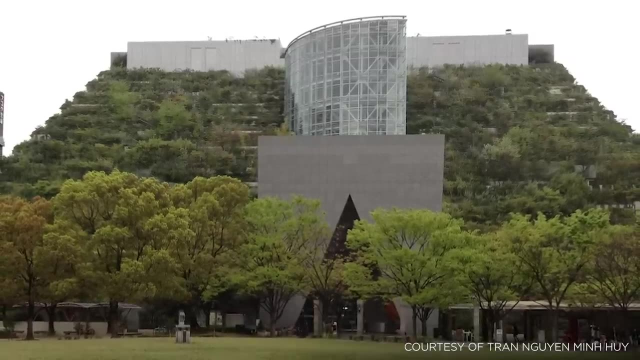 provide enough space for tree roofs to develop. One of the most impressive examples of this is ACROS, a cultural centre in Fukuoka, Japan. First opened to the public back in 1995, this 14-storey building designed by Emilio Embaz. 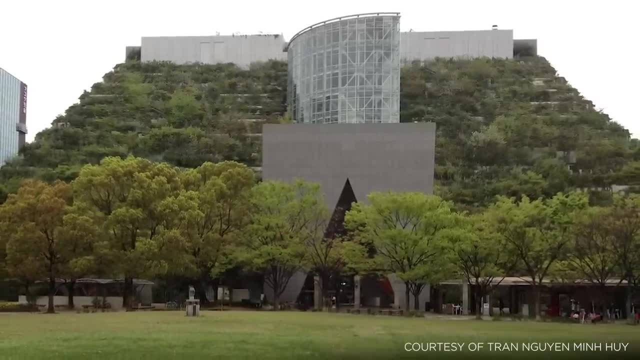 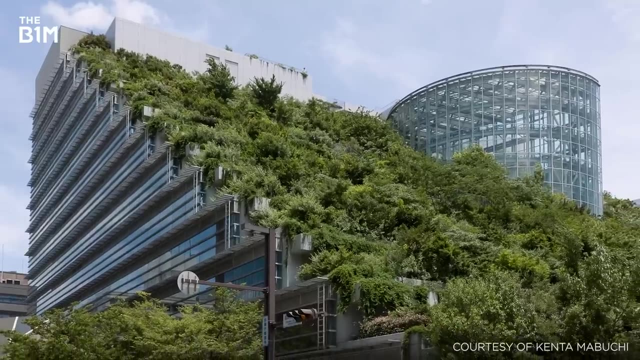 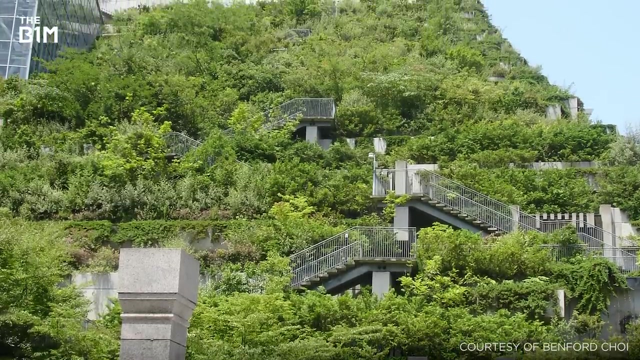 steps down to meet the city's Tenjin Central Park. The building contains deep planters along the edges of its terraces that allow trees to take root and grow. Its 5,400 square metres, or 58,000 square feet of greenery, contained some 37,000 plants. 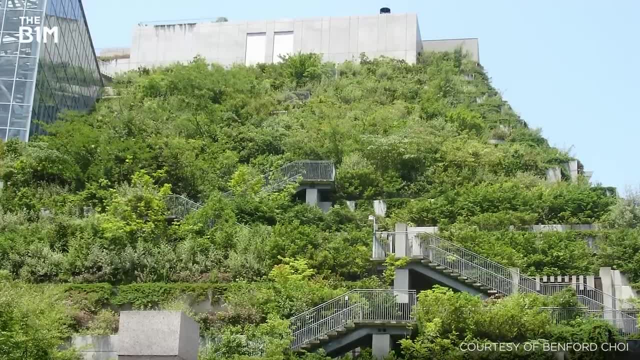 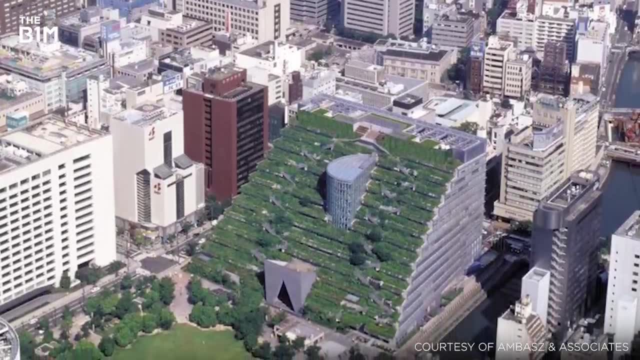 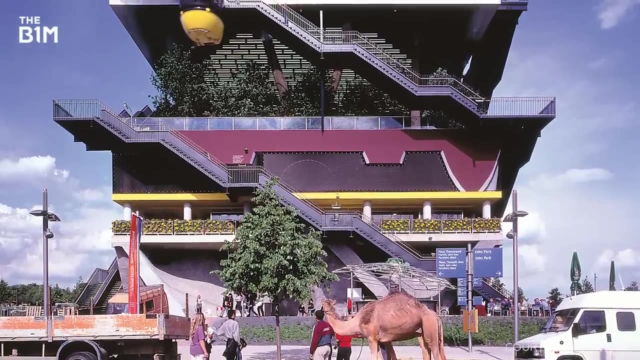 representing 76 different species when it first completed. Conclusion, Conclusion, Conclusion, Conclusion, Conclusion, Conclusion. The Green Roof project also includes more than 120 varieties of plants and over 50,000 individual specimens. Conclusion: Architectural Office MVRDV took a similar approach when designing the Netherlands pavilion. 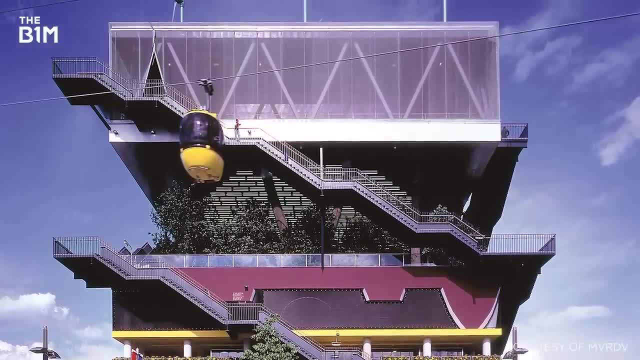 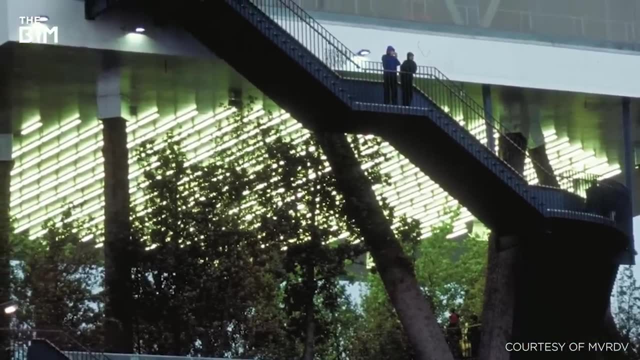 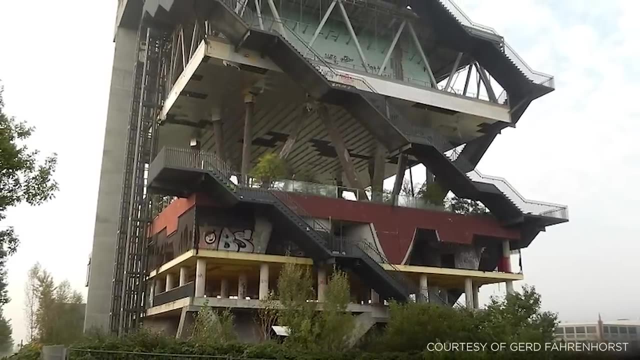 for the 2000 Expo in Hannover, Germany. Here, the entire fifth floor of the structure was given over to a forest in which deep planters accommodated mature trees. Conclusion. Conclusion: since fallen into disrepair, with the mature trees dying off a new generation of shrubs. 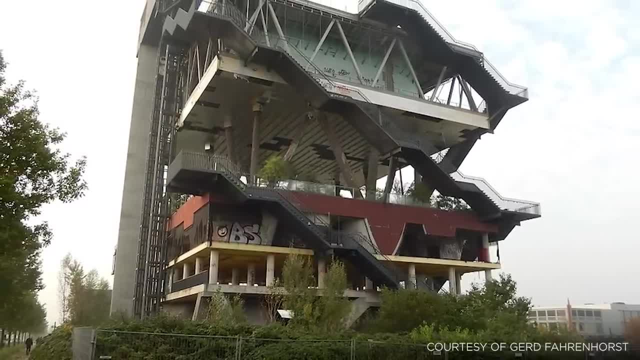 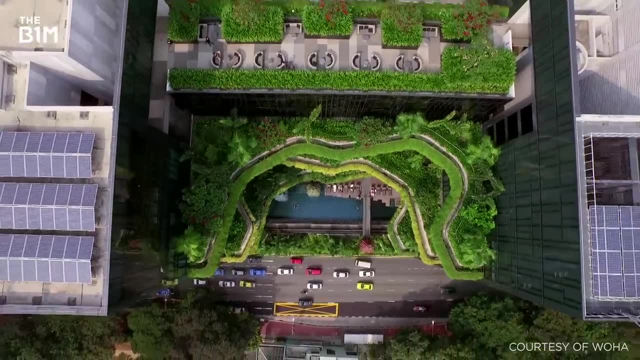 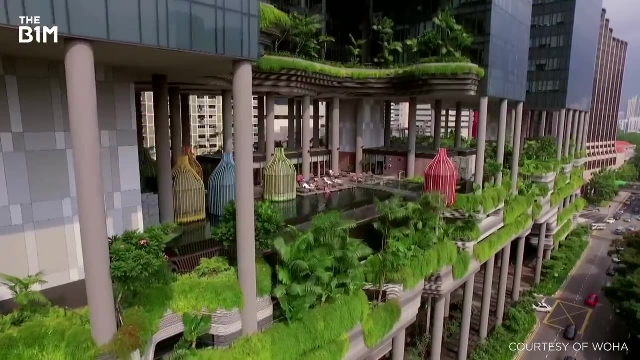 and trees has since colonised the structure, proving the soundness of the principle. Later in the decade, architecture and engineering firm Wohar designed the Royal Pickering Hotel in Singapore, which included extensively planted terraces at four-storey intervals, featuring. 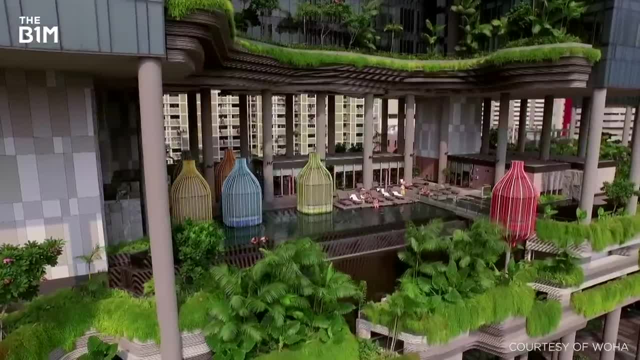 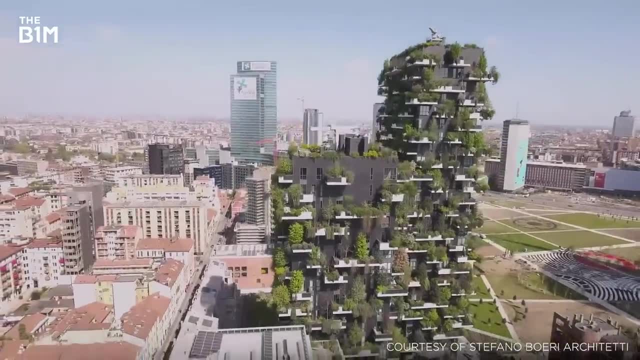 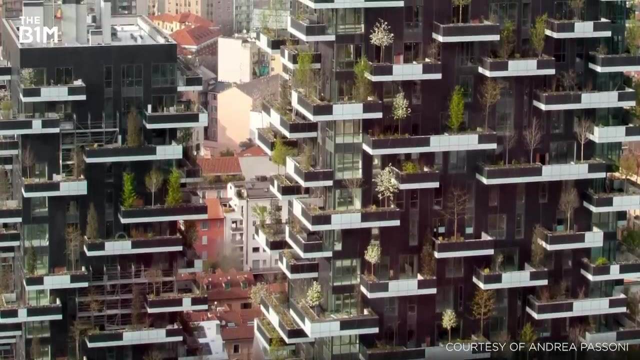 tropical shrubs, vines and palm trees. This building, completed in 2013,, just a year before the twin towers of Bosco Verticale, or the Vertical Forest in Milan, Conceived by Stefano Boeri architects, these residential towers standing 112 metres and 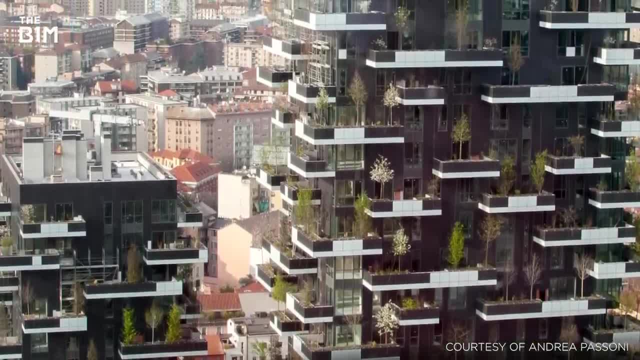 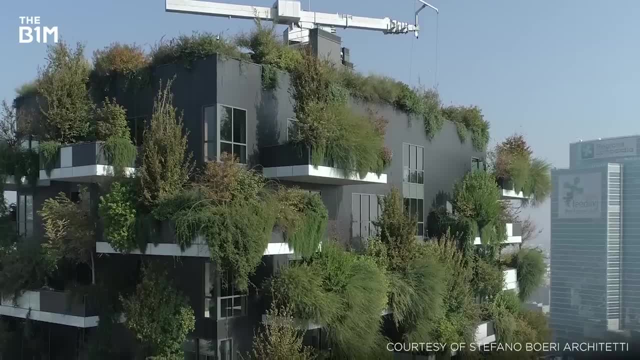 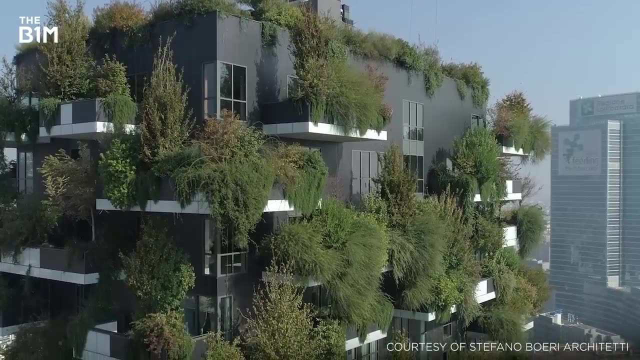 76 metres tall respectively, in central Milan are the first successful example of tall buildings fully covered in trees Standing between 3 and 6 metres tall when they were first planted. the trees will be allowed to reach a maximum height of 9 metres before being pruned. 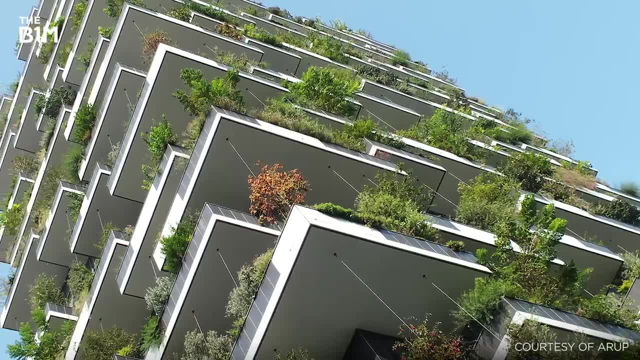 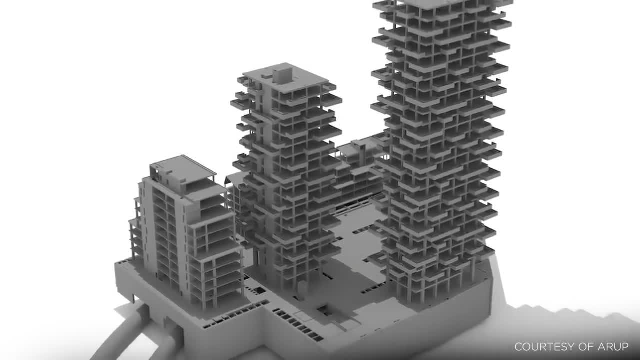 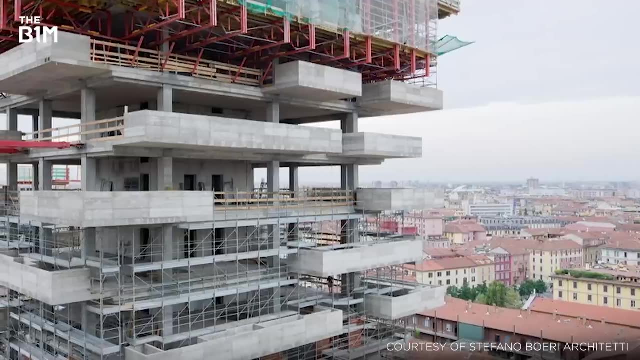 In order to ensure their stability in the wind, the trees are tethered to the building using steel wires. Structurally, buildings that incorporate trees will, of course, require special consideration and additional strengthening and reinforcement in areas. In the case of Bosco Verticale, the additional 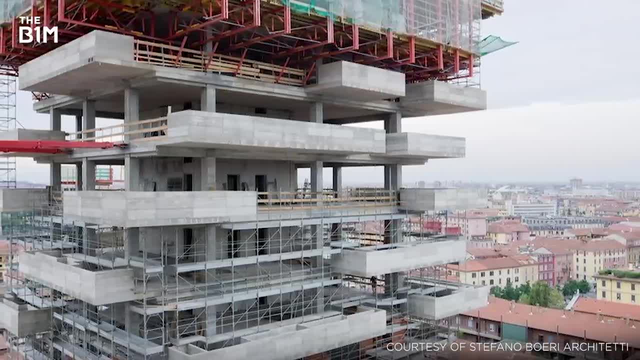 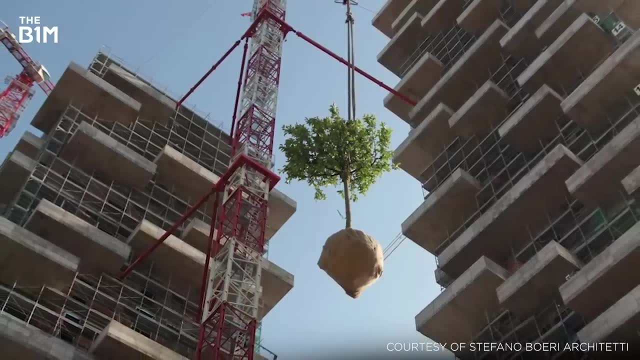 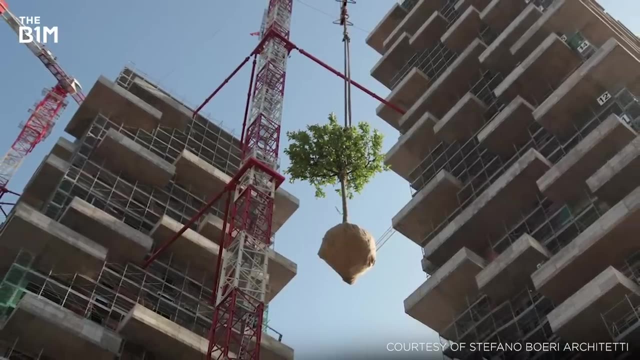 cost of this reinforcement was clearly offset by benefits and did not prevent the project proceeding. There are other issues to consider when mixing trees with buildings too, such as the embodied carbon of the steel used in reinforcement or building superstructures and the increased demands placed on maintenance. 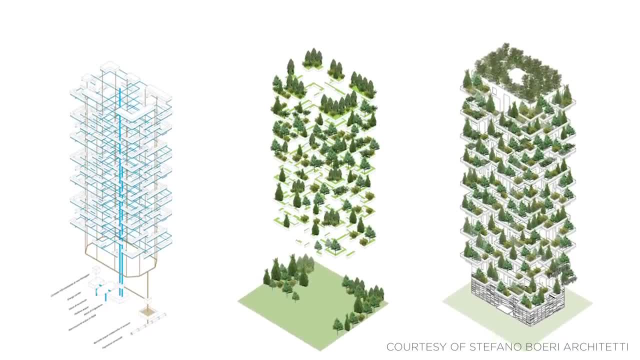 In this example, the project team were able to use Milan's excess underground water to cultivate the trees, minimising the tower's ecological footprint. In this example, the project team were able to use Milan's excess underground water to cultivate the trees, minimizing the tower's ecological footprint. 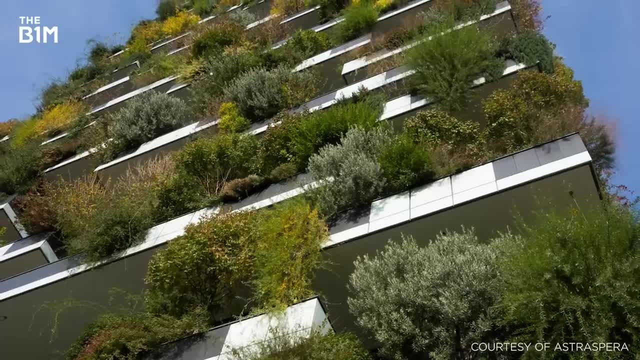 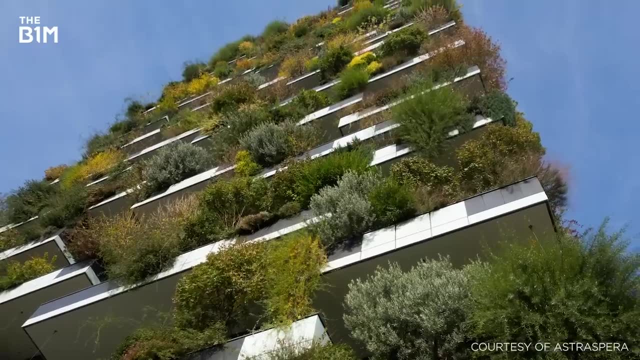 In this example, the project team were able to use Milan's excess underground water to cultivate the trees, minimizing the tower's ecological footprint. Another challenge posed by this new building type, with large amounts of potentially flammable organic matter attached to facades, is fire. 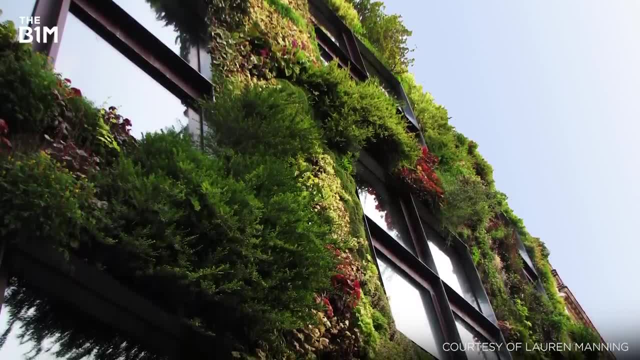 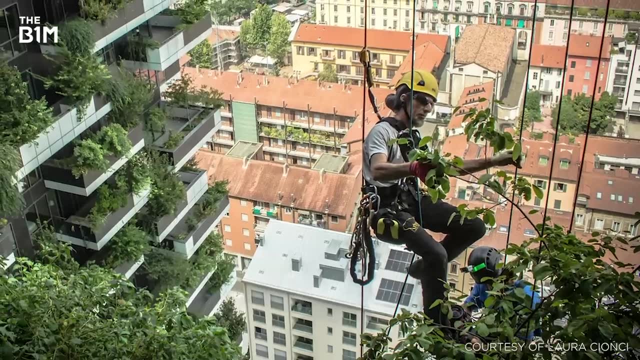 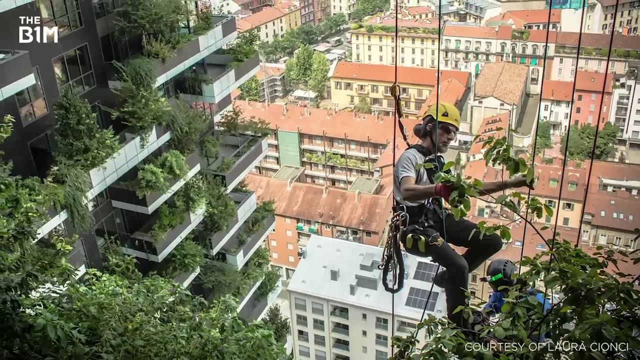 Principally, engineers use established guidelines for green facades and green roofs to ensure their buildings meet fire safety regulations. Regular pruning and irrigation also help to mitigate the risk of fire, as does ensuring that the soil contains a relatively low percentage of organic matter. 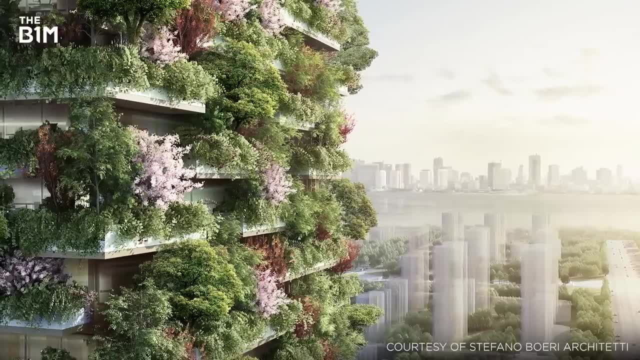 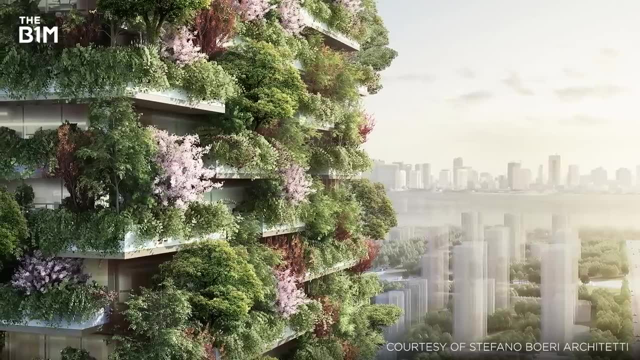 Regular pruning and irrigation also help to mitigate the risk of fire, as does ensuring that the soil contains a relatively low percentage of organic matter. Learning from his work in Milan, Stefano Boeri is currently working on a number of similar projects in places such as Switzerland, China and the Netherlands. 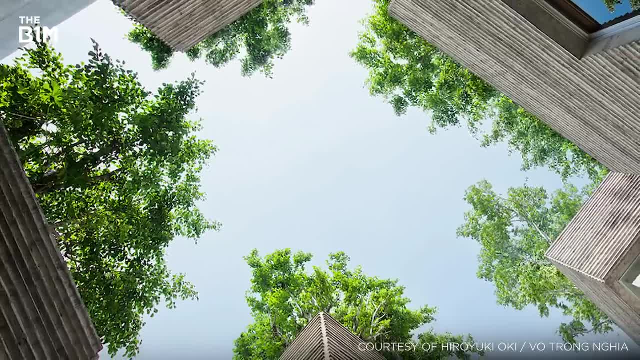 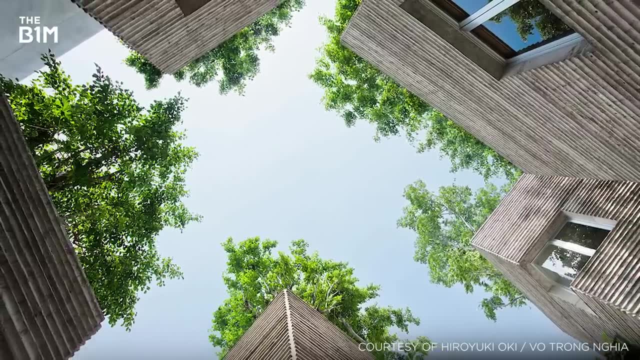 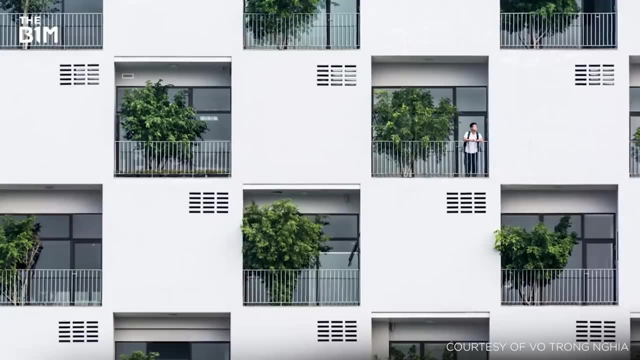 The concept of incorporating trees into buildings is also employed across Southeast Asia and features heavily in the work of Vietnamese studio Vo Truong Nghia, who have incorporated trees into buildings as diverse as private rooms. The project includes building as diverse as private residences through to a university office in Hanoi. 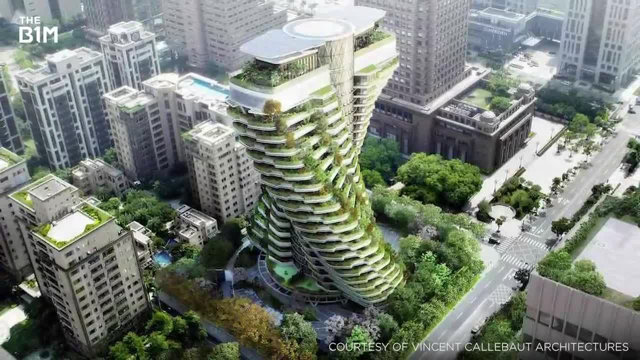 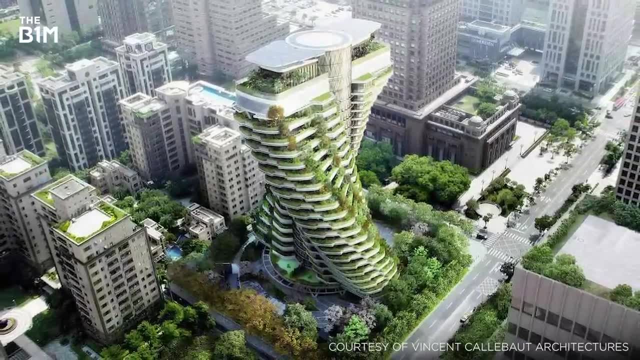 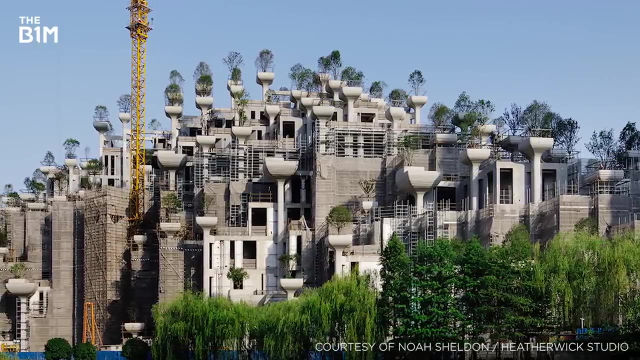 Currently under construction in Taipei, Belgian architect Vincent Callebaut's Agora Tower, based on the form of a DNA double helix, will feature extensively planted balconies. Meanwhile, in Shanghai, British designer Thomas Heatherwick's 1000 Trees, a mixed-use building. 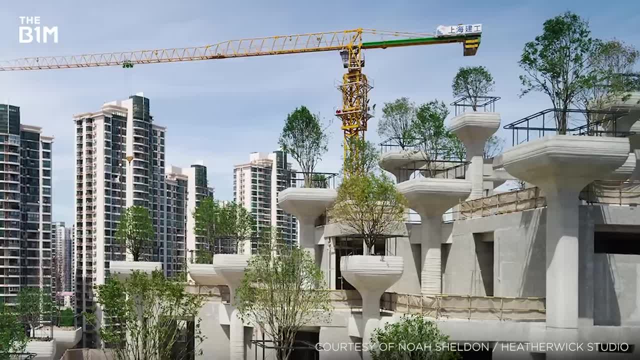 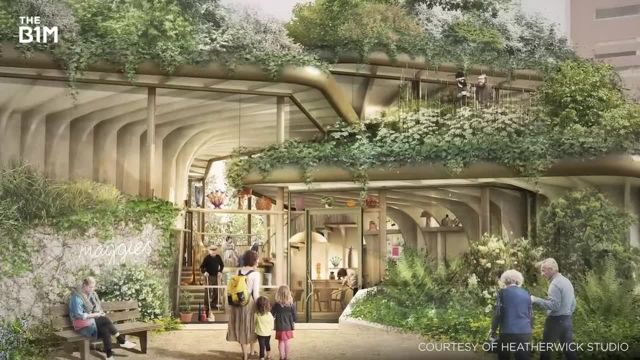 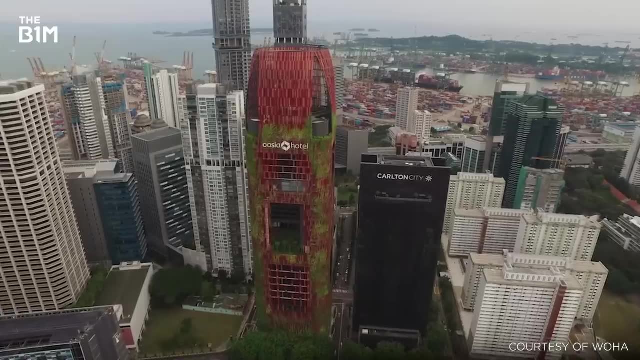 that features trees and shrubs on its structural columns is nearing completion And in the UK, Heatherwick's Maggies Centre in Leeds uses its roofs to create a stepped garden complete with trees and lush vegetation. In Singapore, Wohar continue to design green architecture, including the Oasia Hotel downtown.